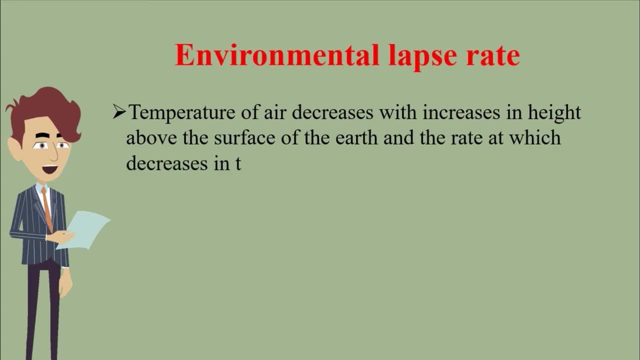 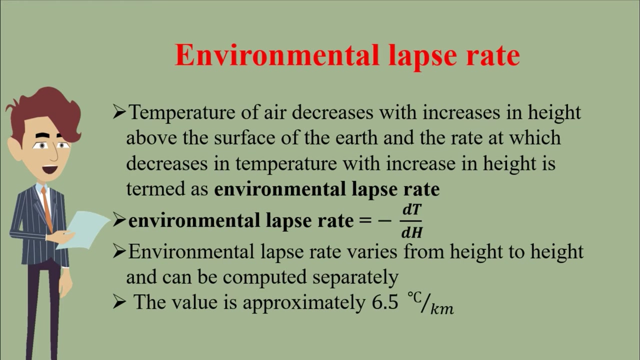 the surface of the earth and this rate, at which decrease in temperature with increase in height, is termed as environmental lapse rate. Environmental lapse rate is equal to minus dt by dh. Environmental lapse rate varies from height to height and can be computed separately, and this variation is approximately equal to 6.5 degree centigrade per kilometer. And. 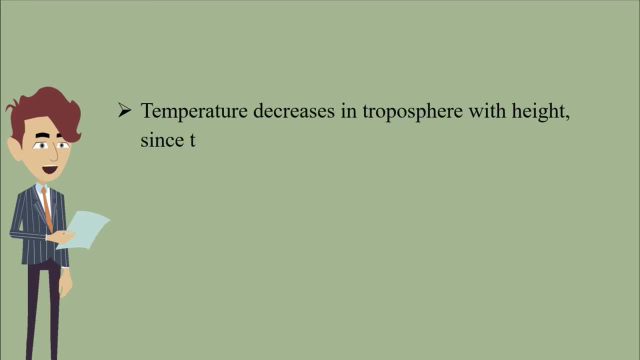 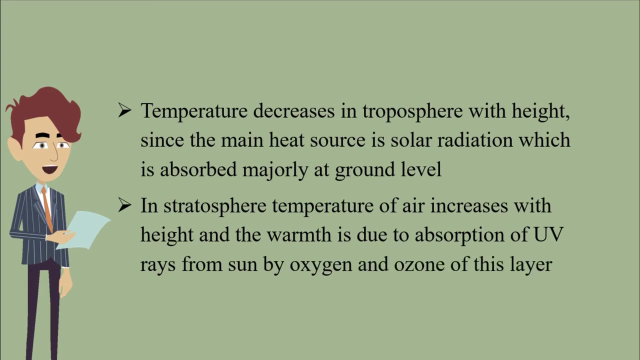 the temperature decrease in troposphere with height, since the main heat source is solar radiation, which is observed majorly at ground level, Whereas in stratosphere the temperature of air increases with height and the warmth is due to absorption of UV rays from sun by oxygen and ozone present in this stratosphere. Now we will learn about the temperature of. 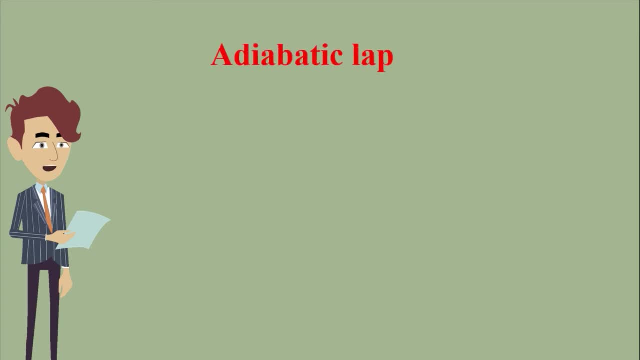 air. Let us learn about adiabatic lapse rate. What is adiabatic lapse rate? When pollutants rises into the atmosphere, its temperature also decreases with increase in height, at the expense of its internal energy to carry out its expansion. while rising into atmosphere, The rate of 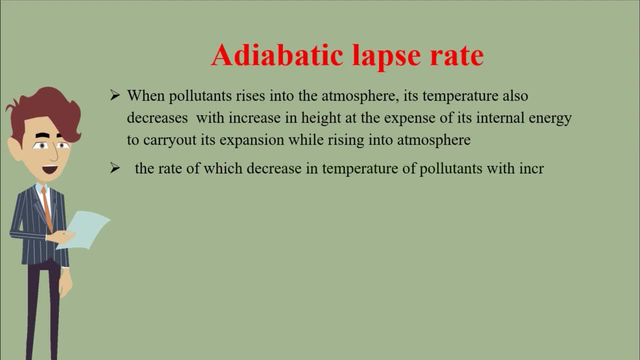 which decrease in temperature of pollutants with increase in height, is termed as adiabatic lapse rate, And the adiabatic lapse rate depends upon the moisture content present in air. For wet air, the adiabatic lapse rate is 6 degree centigrade per kilometer and for dry air adiabatic lapse. 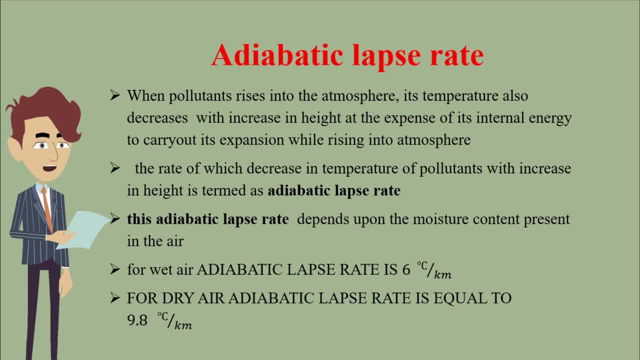 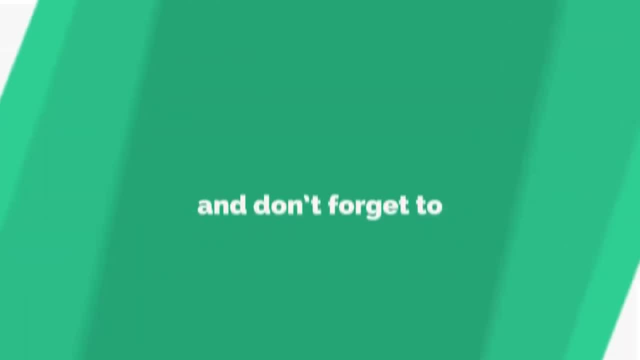 rate is equal to 9.8 degree centigrade per kilometer And the adiabatic lapse rate is equal to 9.8 degree centigrade per kilometer And the adiabatic lapse rate is equal to 9.8 degree centigrade per kilometer. And the adiabatic lapse rate is equal to 9.8 degree centigrade per kilometer.